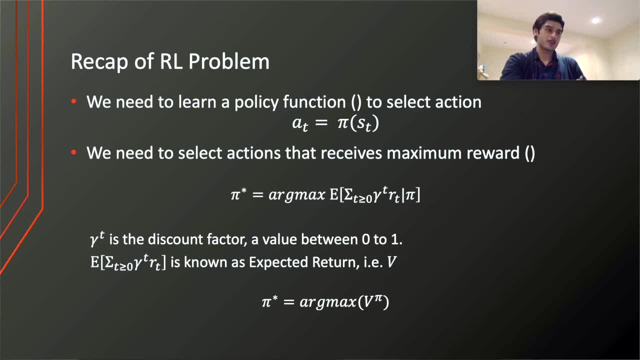 for that given policy and that gives us our optimal policy as defined by this equation. Now here v, which is the value function, is basically known as a state value function, which is which gives us the expected return for starting at some particular state s and then always following. 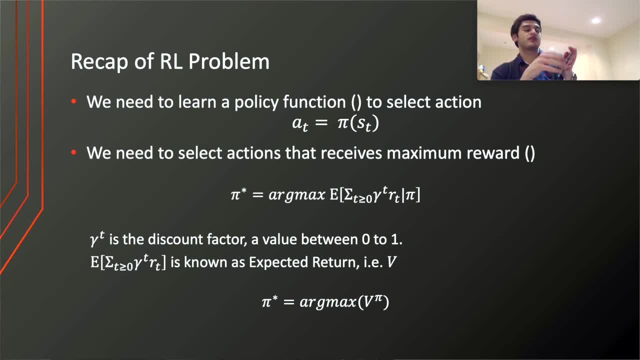 policy pi. So this actually expects this function requires that we follow some policy that we already have. but the problem in our scenario is we don't actually have a policy because our neural network hasn't learned anything. Initial functions that the neural net will take will essentially be: 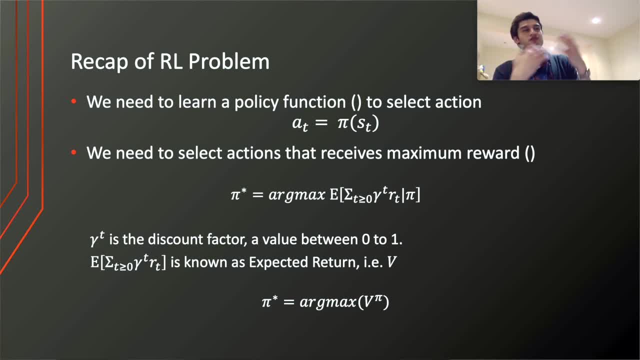 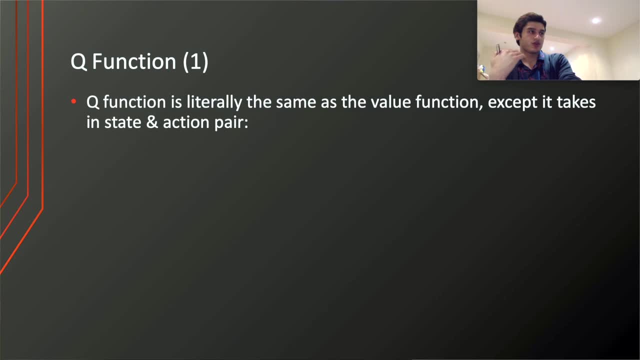 random. So we actually need a different value function that accommodates our needs. So we introduce what is known as a q value function, which is a value function that accommodates our needs, And what it takes in is the state action pair, and it is. it basically defines the expected return. 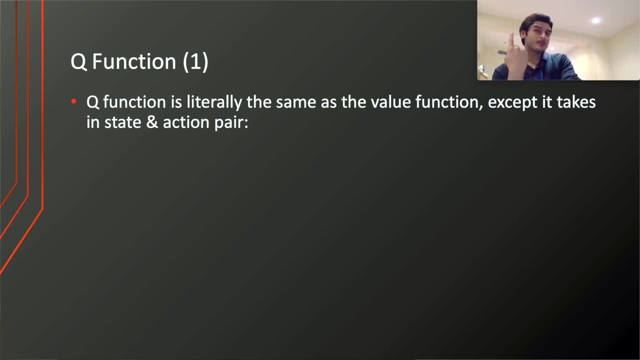 starting at some state s, but then taking an arbitrary action a, and this action a does not necessarily have to come from a policy, since it's arbitrary, so it can be random, But there on after we have to act according to some policy. So we have to take an arbitrary action a and then we have to act according to some policy. 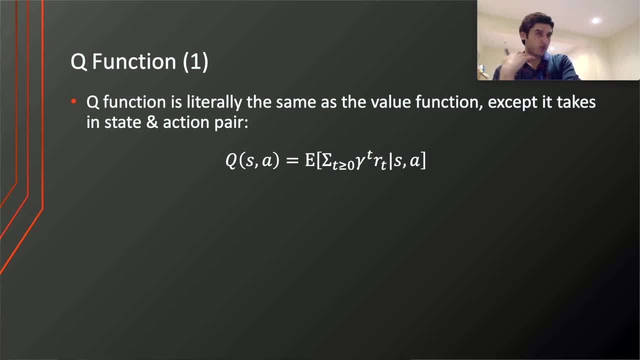 So initially our network will take random actions, but after it has actually wracked up some experiences and we learn from those experiences, we actually have some policy. even though that policy will be weak, we have something. so the q value function or action value function is what we use in the dqn. 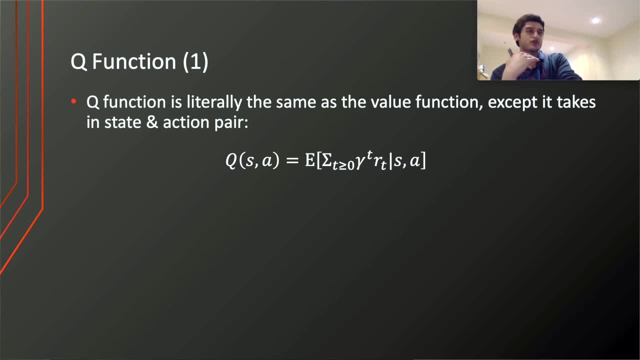 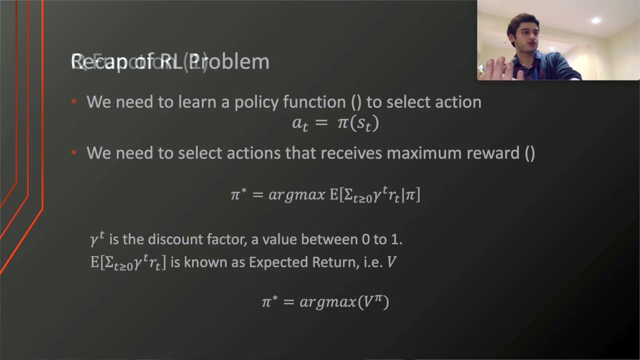 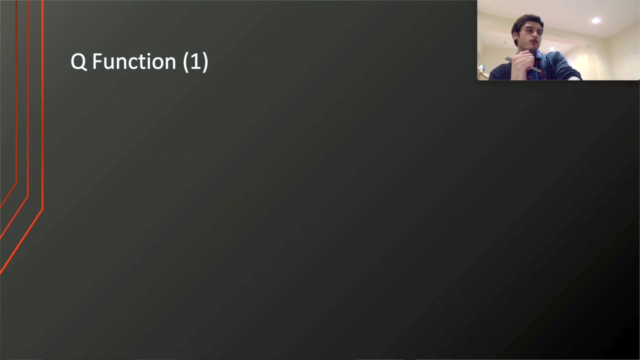 and this, essentially, can be substituted for the state value function in the same way. So optimal value function- i mean optimal policy function, sorry- is simply just the maximum of the optimal action value function, similar to optimal policy function being the maximum of the state value function. and what we also know is that these value functions, both state value function, 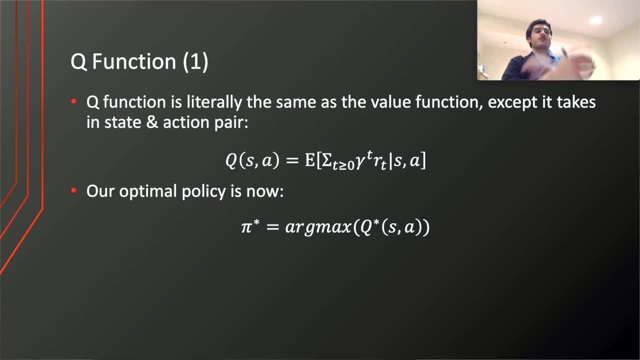 and action value function, but for now let's just focus on the action value function, since that is what we actively use- follows the bellman rule. it obeys the bellman rule. now, proving that mathematically is a whole different problem, and i think we're going to stay clear from that. otherwise, 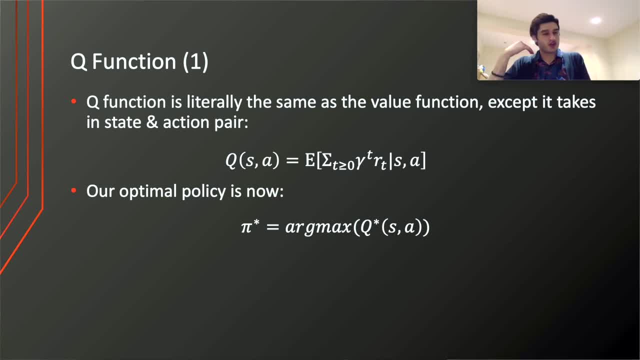 this will take a while, but just i just want you to basically accept the fact that the value function obeys the bellman rule, which is a recursive rule that states that the value of a current state is the reward we get for that particular state, as well as the expected reward. 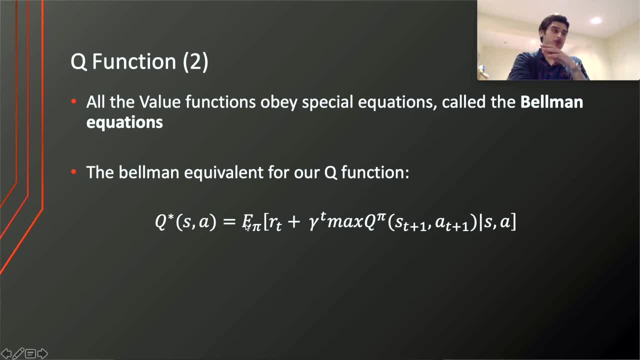 for the successor state, so the expected reward for the next state. so if we actually look at the bellman equivalent of our action value function, then it is exactly as we said. so the optimal q value, or the optimal value for our current state, given some action, is the reward we get for that particular time step, for that particular state, plus the 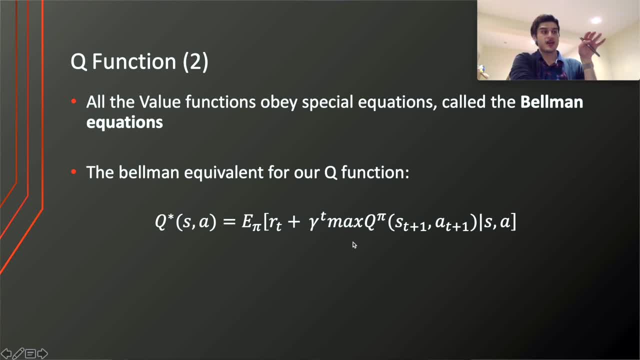 expected value or expected return we get for the next state and the possible action we will take. so that is, that is essentially the bellman equation, and basic idea in reinforcement learning is to estimate this optimal q value by using this bellman as an iterative update, and that's. 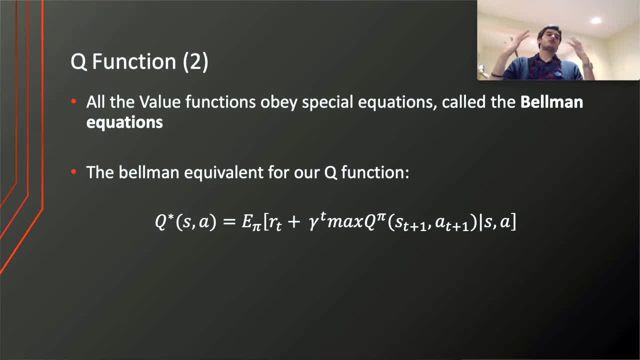 what the value iteration algorithm does. so the value iteration algorithm simply given, given our, the value iteration algorithm simply given, given our experiences which we have stored. let's say you have a sequence of transitions, right state, state action, reward. state action, reward. next state action, reward. next state action, reward, so on. so we have this sequence of state next state, state next state. 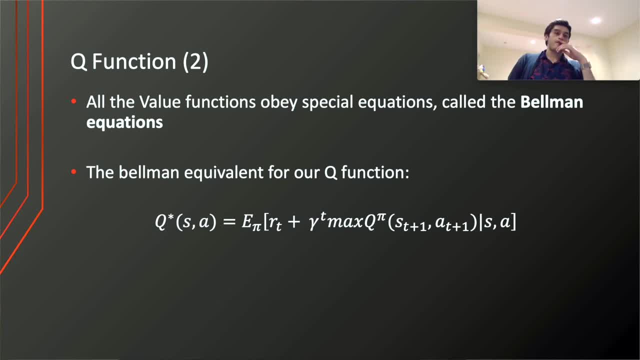 or state, the next state, next state, next state, etc. and the sequence for each of the current state we can expect, we can calculate the expected reward for the next state and therefore the maximum Q value for a given action And therefore we can predict what the next action should be. 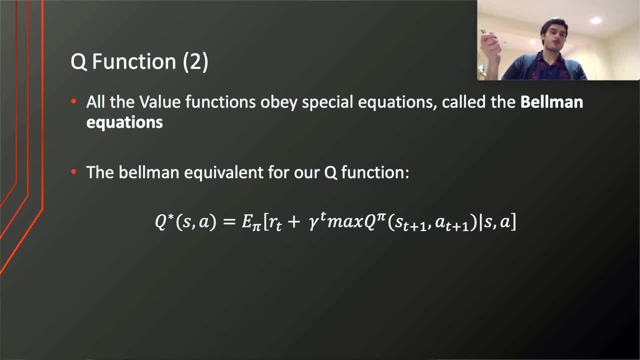 But the problem with this iteration, this iterative algorithm, is that it's actually quite impractical because the Q value from the Bellman update has to be computed separately for each sequence of our experience, for each sequence, So when we actually reinitialize the environment, 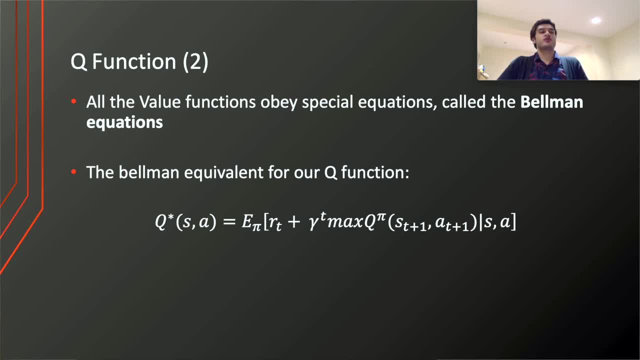 we have to calculate it all over again. So if we were to deploy this in the real world, we would have to have this huge history of sequences from which we would calculate our Bellman expected reward And then, based on that, we would select the optimal policy. 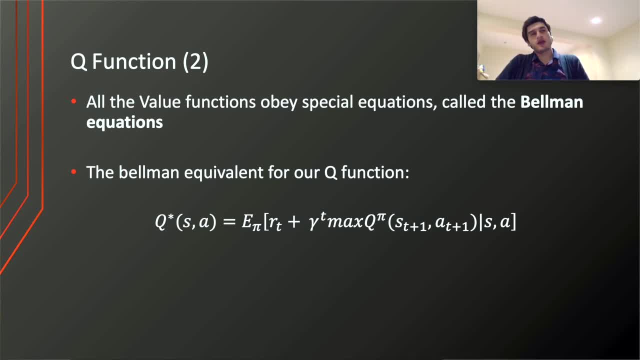 Now that is A inefficient and B, as I said, impractical. So what if we could just learn a function that is able to perform similar to the Bellman equation? So, instead of iteratively doing this, what if we just learned? 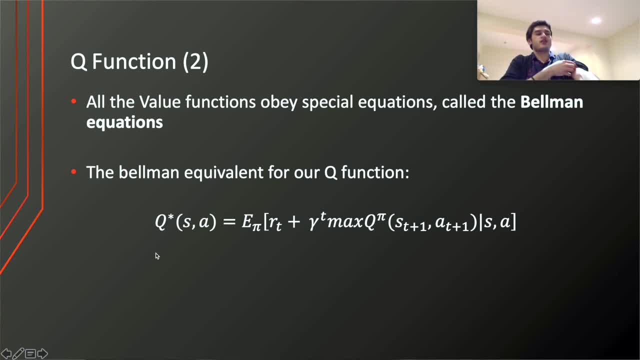 the underlying function that can map our input by learning some features that can give us the output Q value which is similar to the optimal Q value we get from our Bellman output, in which case this becomes a regression problem. So if this is a regression problem, 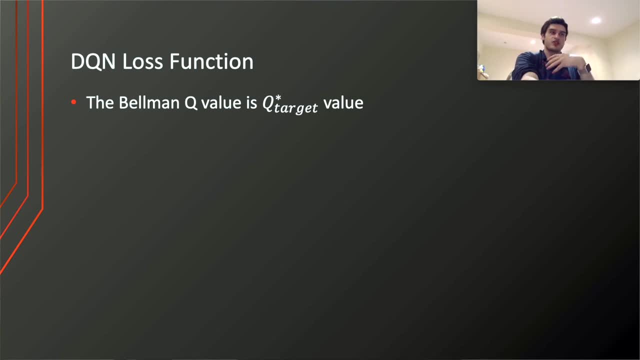 the way we would formulate is is that the Bellman is our target Q value. That is the Q value level we want to obtain And the output of our Q value, our model, which is the Q network. hence the DQN, because we use a deep learning. 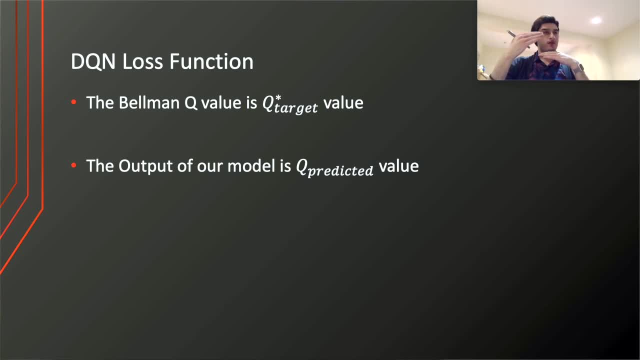 to model that Q network. The output of our network is the predicted Q value for all the possible actions And we want the output of the network, the Q value, to be almost same as the target Q value which we would have got from our Bellman equation. 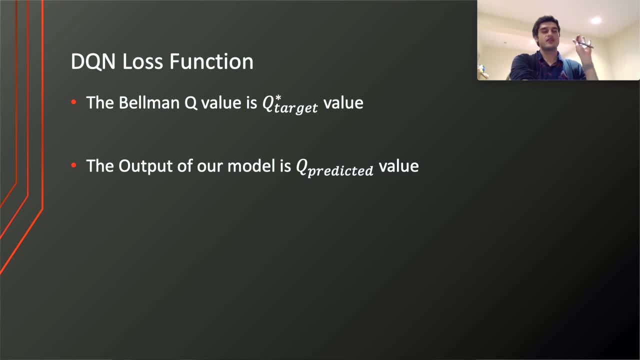 So how can we adjust our weights in our neural network such that the predicted Q value always appears as a Q target value? So you must've seen this when we do linear regression or actually just looking at MNIST classification, right, We could just calculate the distance. 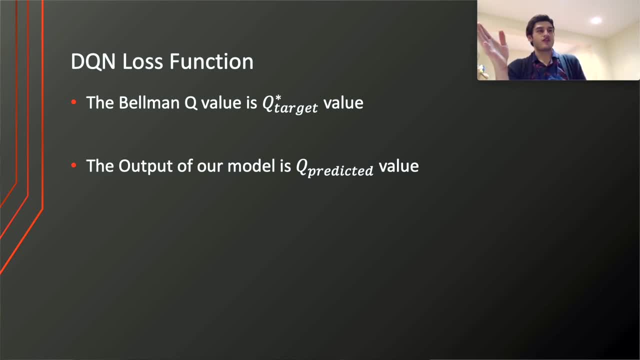 that our output prediction is from our target value, And then we can just back propagate that weights using multivariate chain rule, which is essentially what back propagation is. So we can simply calculate our loss as our mean square error, which is a Euclidean distance between the target Q value. 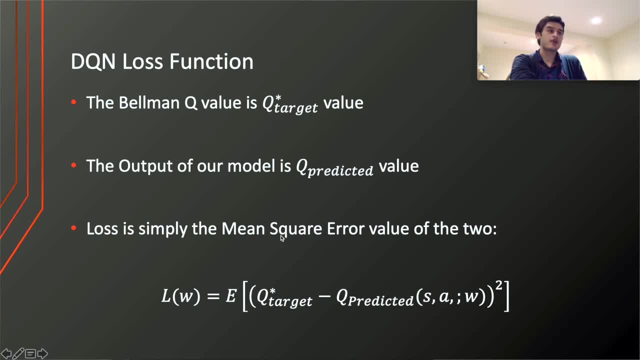 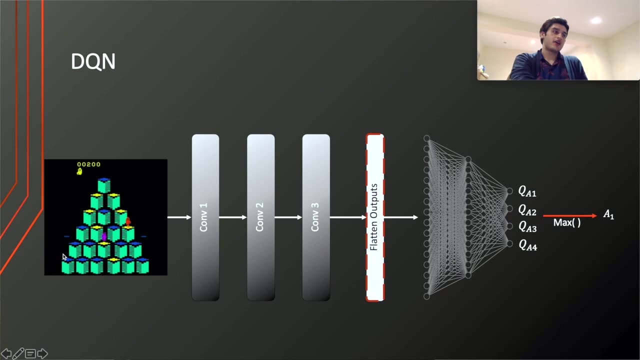 which is, like as I said before, obtained by our Bellman and the Q predicted, which is from our network, And we then back propagate this loss to update our Q network. So if we were to look at an actual scenario, let's say we have an Atari games. 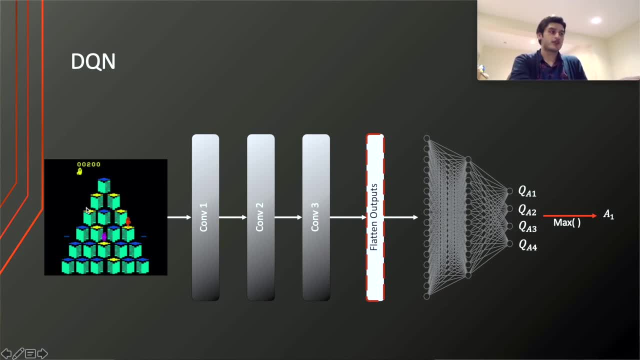 and let's say the total number of actions we can take are four different actions. I mean, I couldn't find the particular screen for an Atari game with four different actions, but let's just say this screen is from an Atari game which we will use as an input. 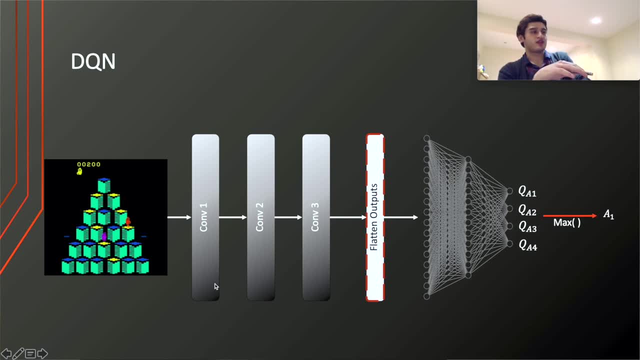 And we will put that in our convolutional neural network, which has three convolutional layers, And then we flatten the output of these layers and then pass it through before we connect it. And the last layer is essentially: each node is associated with the action. 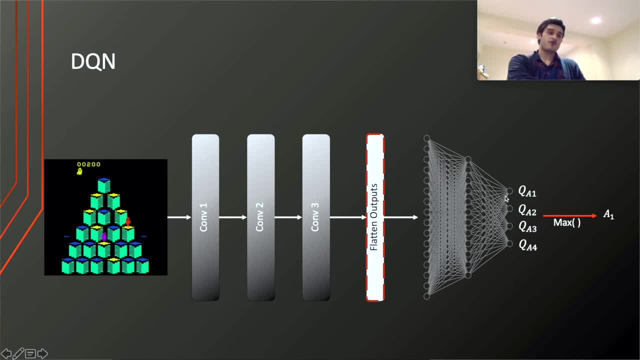 and it will output the Q value for that action. So we have four different actions we can possibly take in this environment, hence four different nodes, And the output is a Q value associated for each action And we select our optimal action as the maximum of these Q values. 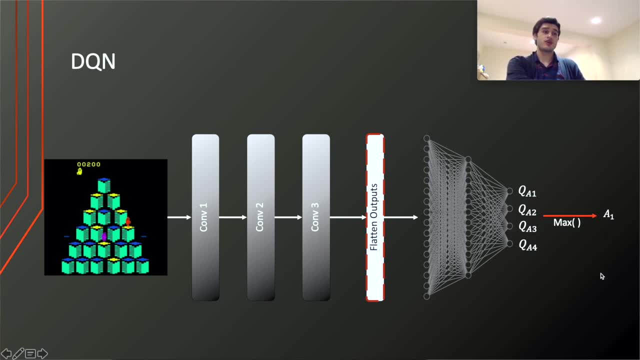 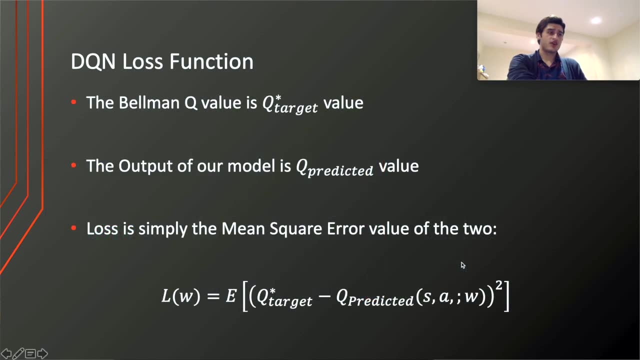 So whichever action node has the highest Q value, we basically use that as our optimal action, as our input to the environment. So if we were to go back to our loss function that we define here, we have our Q predicted value here. So let's say we selected action one. 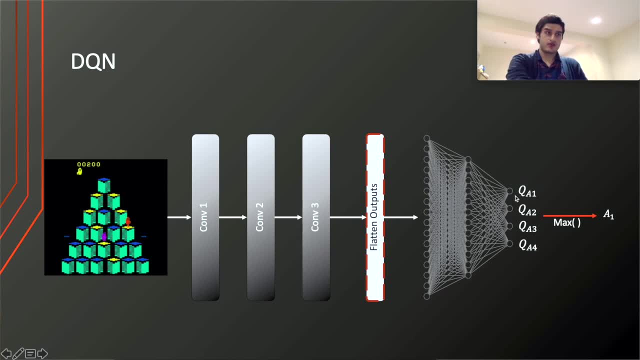 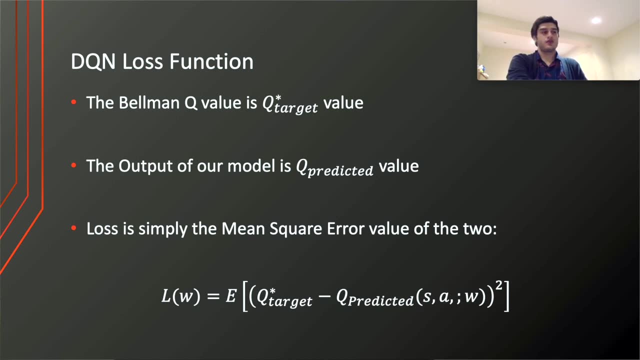 So our Q value for that is QA1.. And then we say, okay, so our Q target for that action, that particular action, is computed by the Bellman- simply do the mean square error and that's the loss we back propagate through the network. 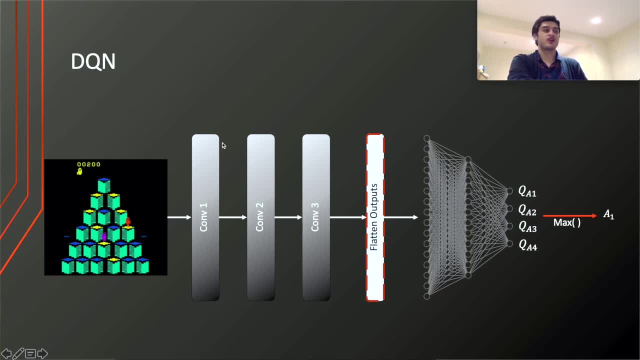 And then we update the whole network iteratively And what we will see is eventually, given enough experiences that we train the neural network with that, the neural network will output Q values associated with all actions given that state, So it is essentially learned the pattern. 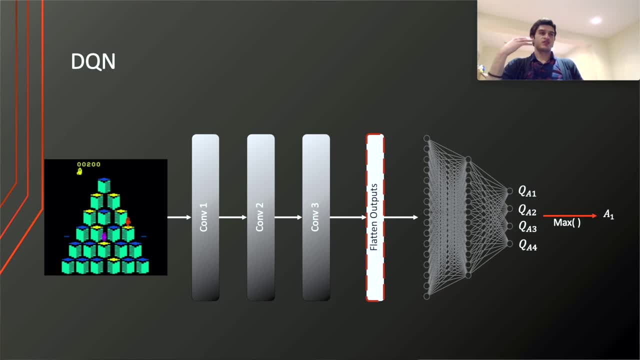 of what the possible Q values should be for the experiences that it has gone through for all the given actions, And then, if we always select the maximum Q value, it will always be the right action to select. So it's a very intelligent way to indirectly propose. 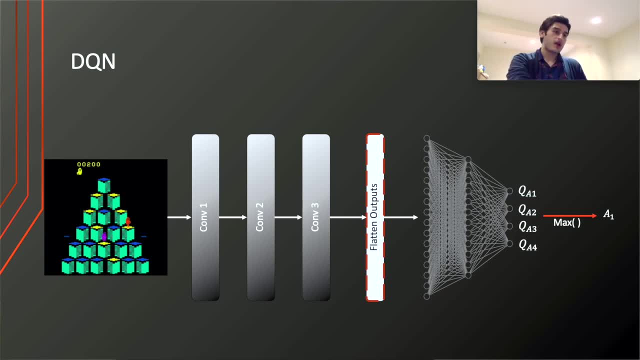 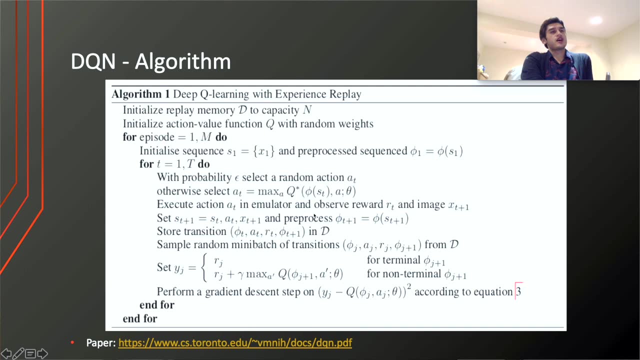 indirectly infer what the policy should be here. So if we actually look at the DQN algorithm which was stated in the paper, this should make more sense now. So we initialize our memory, which is our replay experience, replay memory, so this is where we store our transitions. 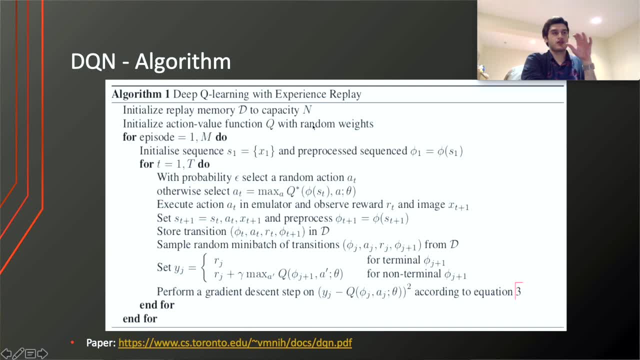 in our experiences And the capacity N is basically up to the user- I think sometimes people go over 10,000 or less. up to you And we initialize our Q network with random weights or you can initialize it with other weight initializers. 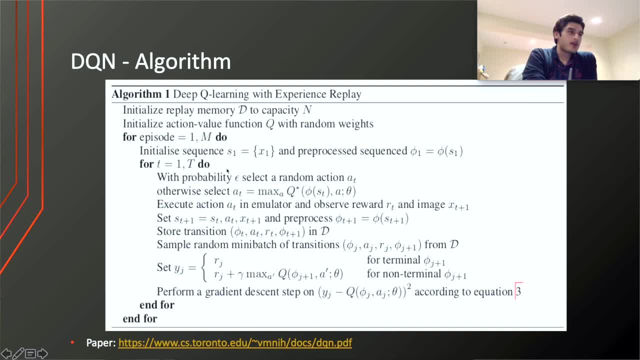 like Xavier or timing, et cetera, And we initialize our environment and we attain our first state by initializing- initializing our environment- And then we select our action. So initially these would literally be random actions, but we can actually select them from our network. 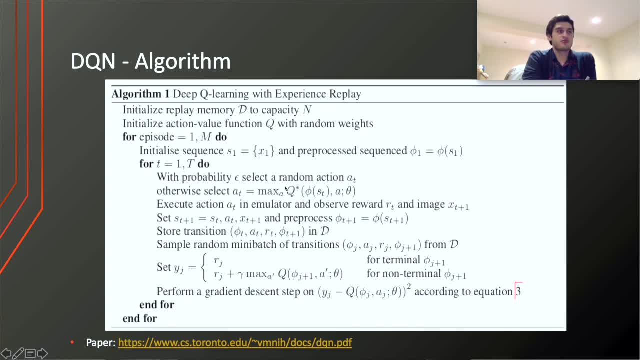 which will be our policy as we learn iteratively And that will be the maximum of our Q output value we get from our network, And that will be the action we select. We simply then implement the action into the environment to get our reward and our next state. 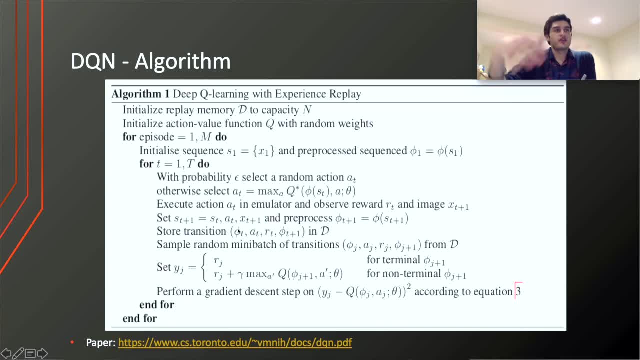 And then we store that state action reward, next state into our transition replay, play memory D. And then we basically calculate the Bowman error, for well, not the error, sorry, the Bowman equivalent, the Q value, Bowman Q value for our state. 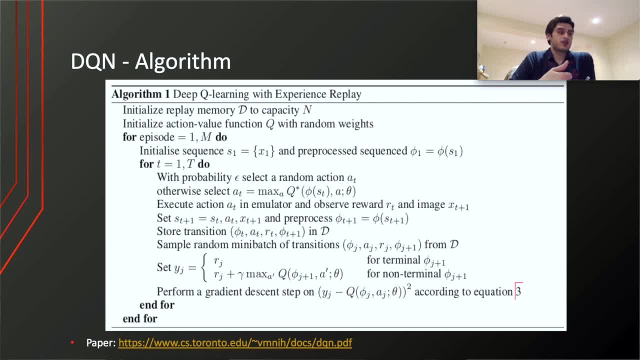 for the current state because we already have our next state. So we calculate the Bowman Q value and that becomes our target Q value which we want to reach. And then we perform gradient descent because we want to minimize the mean square error. 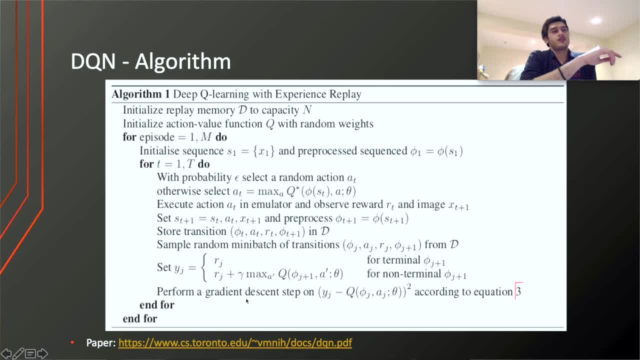 Yeah, We want to minimize the mean square error by taking the gradient step down the loss function by the formula that was depicted in the previous slides, And we keep doing this iteratively till, basically, we've reached a global minimum of our loss function And at that point, 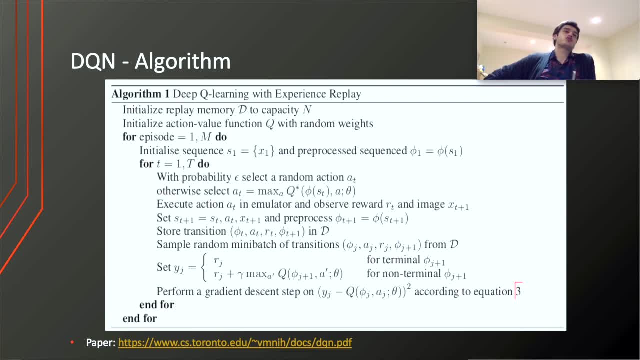 our network will always output the right Q values for our given actions. And that is really it. So, essentially, what we do is we boil this reinforcement learning problem into a simple, simple regression problem by approximating a function, by actually defining a function that approximates. 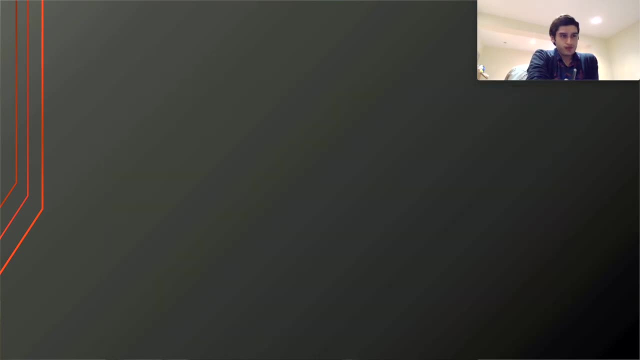 the Q value for the given actions. So that's really it. That's all BQN is. It's basically taking the reinforcement learning algorithm and putting it as a regression problem to predict the right Q value, And then we simply select our actions as the maximum Q value. 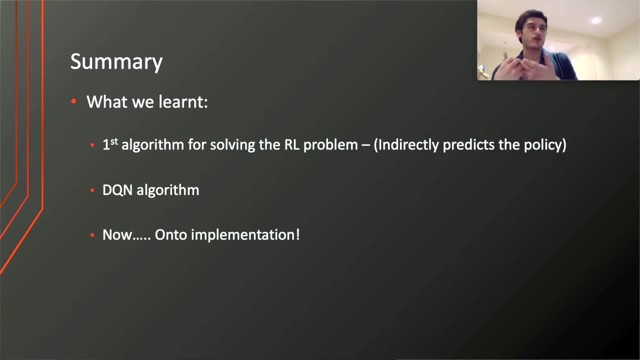 which is our action, associated with the maximum possible reward it can attain for that particular state, And that's the BQN algorithm. It's still a bit difficult to understand, I think after you go through the code which I will upload and the link would be provided in the description below.